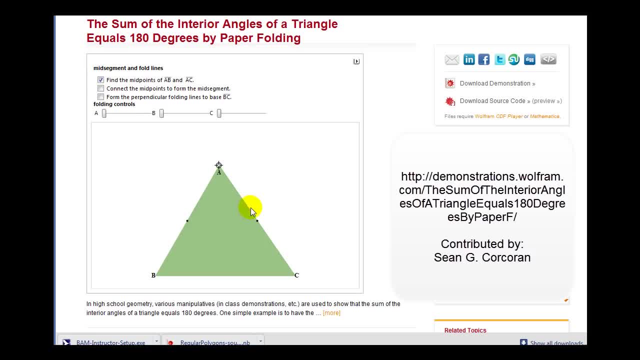 of side AB and side AC. they would be here If we connect the mid segment. we would have this, And then we'll construct the perpendiculars from these midpoints to the base. And now we'll make folds across these segments: One, two, three folds. 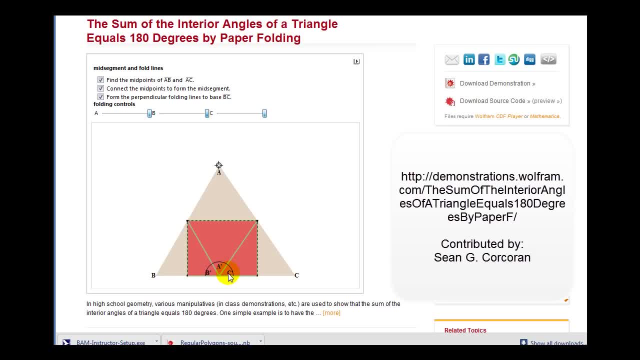 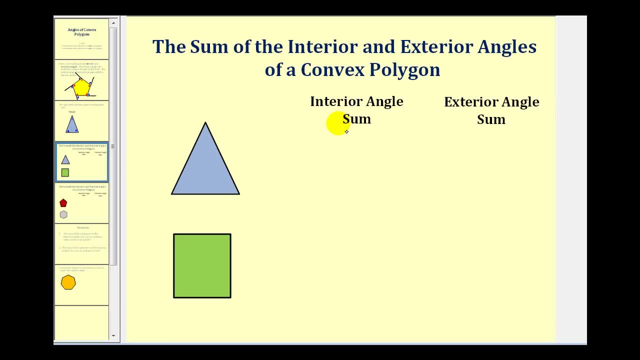 And now we can see very clearly that angles A, B and C would form a straight angle or would have a sum of one hundred eighty degrees. So let's use that information to determine the sum of the interior and exterior angles of some convex polygons. So for this first triangle we know the sum of the. 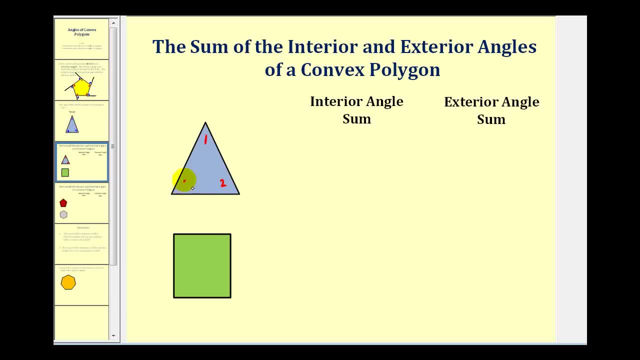 interior angles, angle one, two and three would be one hundred eighty degrees. Now let's go ahead and label the exterior angles, So we'll extend each side, starting here, And so the exterior angles would be angle four, five and six. Well, the sum of the interior and exterior angles 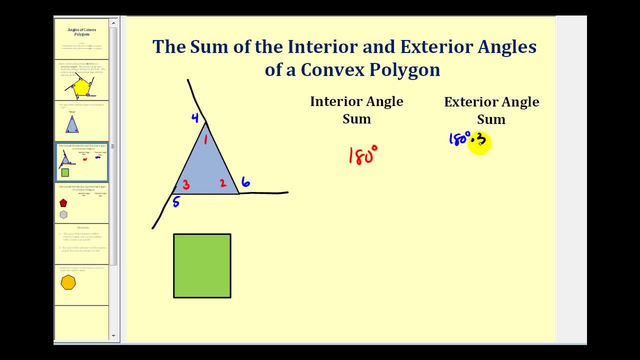 would be one hundred eighty degrees times three. Since angles one and four, three and five and two and six form linear pairs, we know their sums would be one hundred eighty degrees. So this would give us five hundred forty degrees, And if we subtract out the sum of the interior angles, 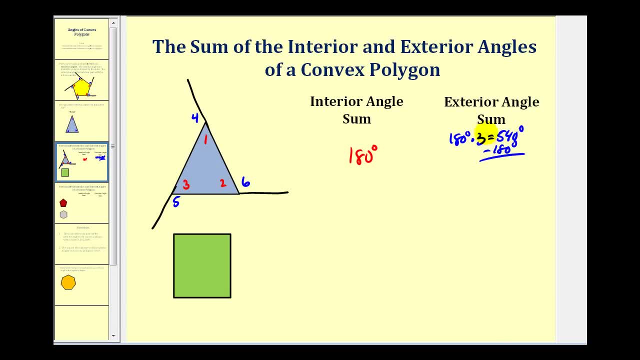 or one hundred eighty degrees, we'd have the sum of the exterior angles. That's going to give us three hundred sixty degrees. Now for the interior angles of a quadrilateral. we're going to break up the interior into triangles, since we know the sum of the 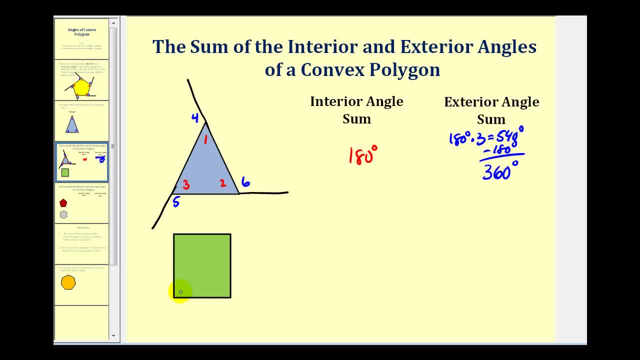 interior angles of a triangle would be one hundred eighty degrees. Using that logic, we can see that there would be two triangles in the interior of a square, and therefore the sum of the interior angles would be one hundred eighty degrees times two or three hundred sixty degrees. 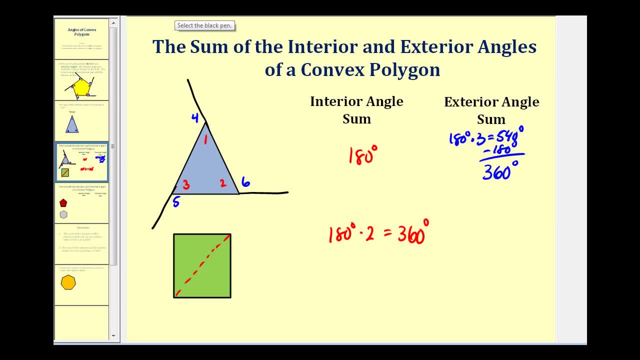 And then, when it comes to the exterior angles, we'll go ahead and extend each side. So if we label the interior angles and the exterior angles, the interior and exterior angles make up four linear pairs. So the total sum would be one hundred eighty degrees times four. 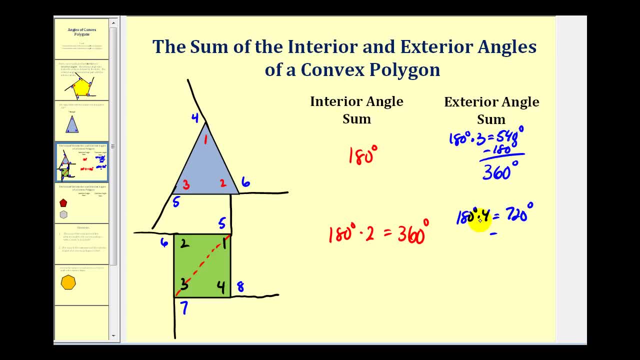 It's going to be seven hundred twenty degrees, And if we subtract out the sum of the interior angles, which is three hundred sixty degrees, we would have three hundred sixty degrees as the sum of the exterior angles. So notice how the sum of the interior angles is changing. 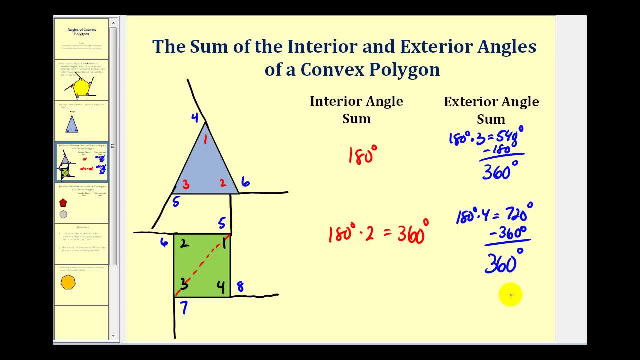 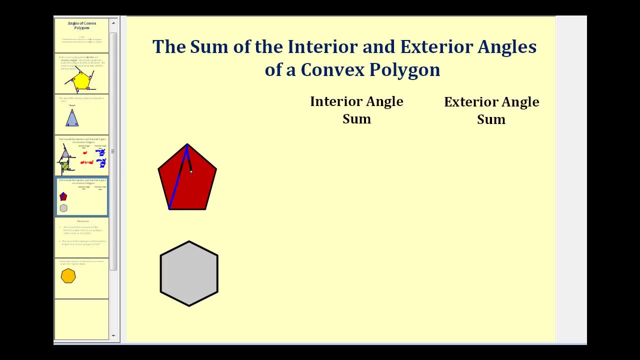 but the sum of the exterior angles is staying the same. Let's go ahead and try at least one more. For the pentagon, we can divide the interior into three triangles. Therefore, the sum of the interior angles would be one hundred eighty degrees times three, or five hundred forty degrees. 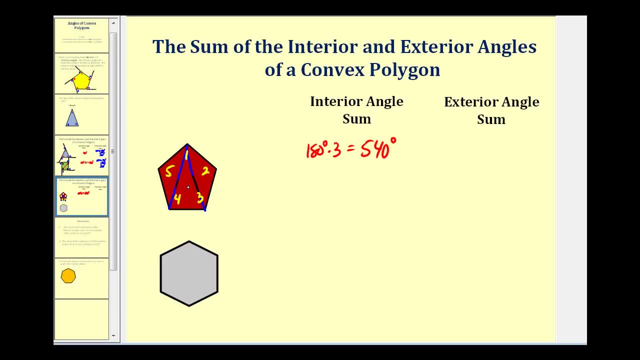 And if there are five interior angles, it would be five exterior angles. So we'd have five linear pairs. So the sum of the interior and exterior angles would be one hundred eighty degrees times five. It's going to be nine hundred Subtracting out the sum of the interior angles. 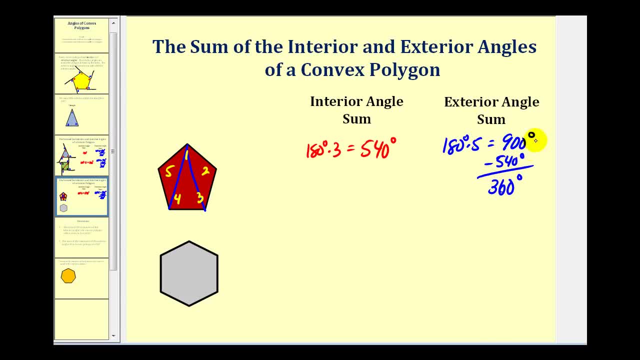 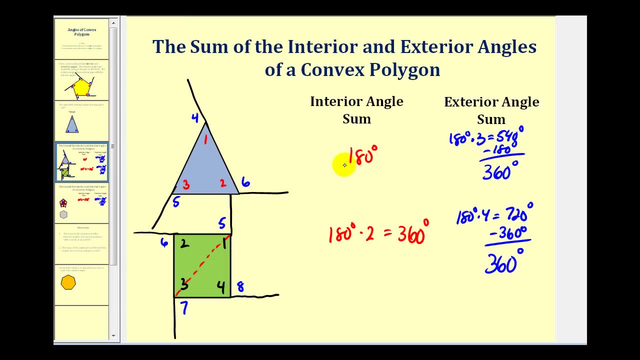 again leaves us with three hundred sixty degrees. So once again, notice that some of the interior angles is increasing, while the sum of the exterior angles stays the same. Let's go back and see if we can notice a pattern. Notice that the polygon has three sides. We can think of this as one hundred eighty times one. 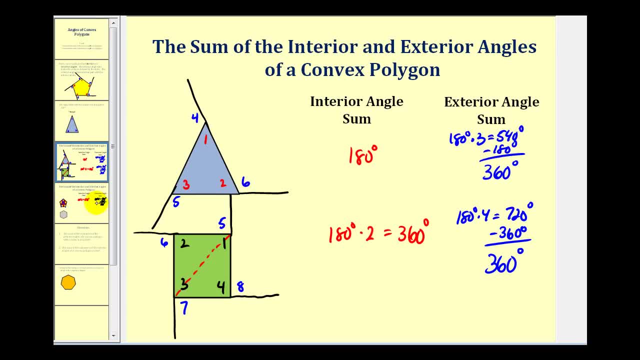 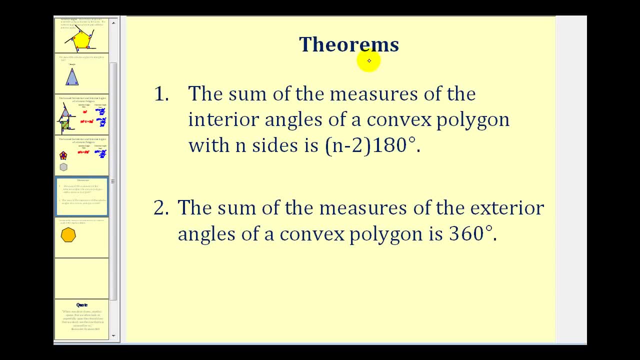 For four sides we have one hundred eighty degrees times two, And for five sides we have one hundred eighty degrees times three. So you probably can see the pattern which leads us to the following theorem: The sum of the measures of the interior angles of a convex polygon. 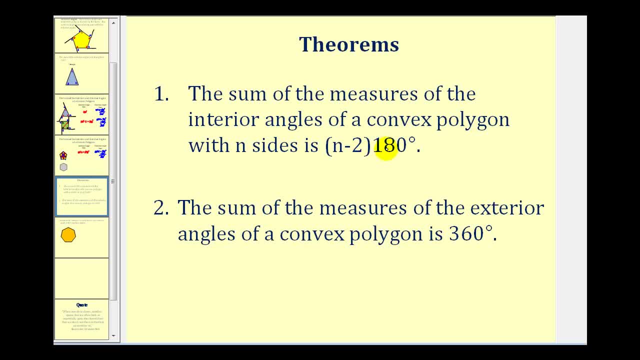 with n sides is n minus two times one hundred eighty degrees. So we take the number of sides subtract two, multiply by one hundred eighty degrees and it gives us the sum of the interior angles And the sum of the measures of the exterior angles of a convex polygon. 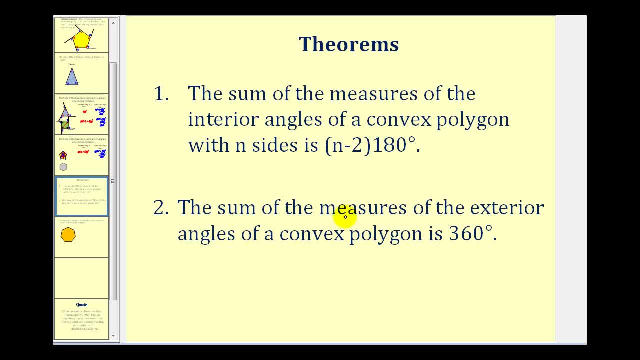 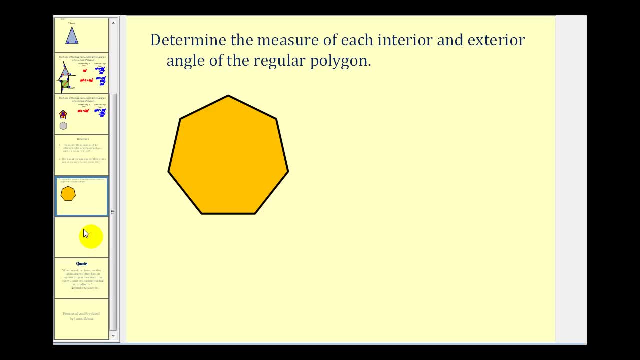 is always three hundred sixty degrees. Let's take a look at an example using these theorems. Here we want to determine the measure of each interior and exterior angle of this regular polygon. Remember, if it's regular, the lengths of all the sides and the measure of all the interior angles are equal. 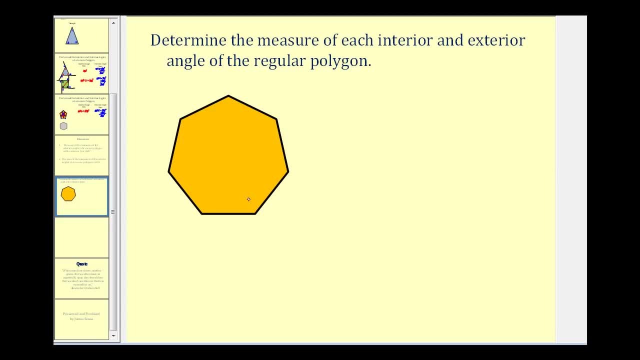 So let's first count the number of sides. we have One, two, three, four, five, six, seven. So it's a heptagon, and n is equal to seven. So we'll start by finding the sum of the interior angles.